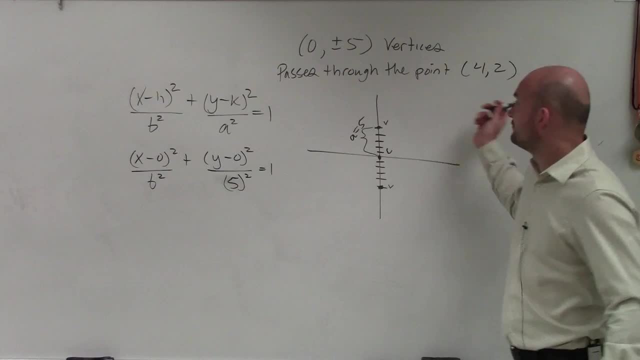 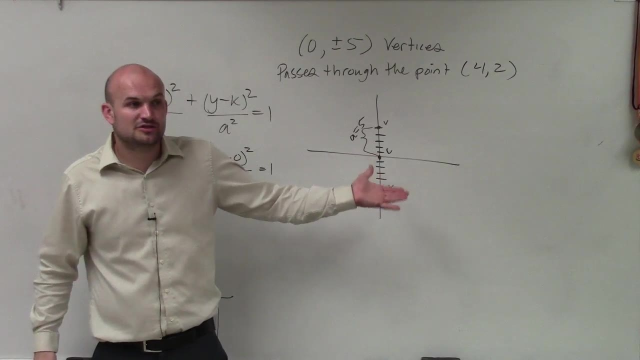 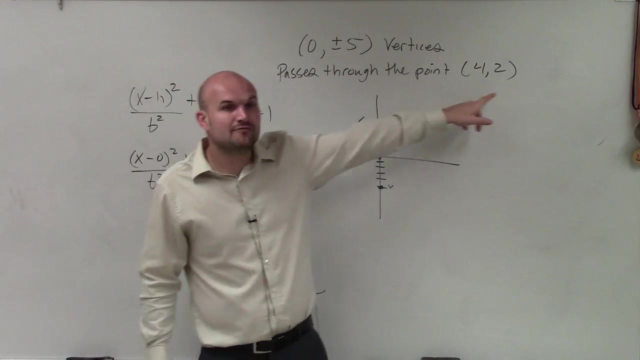 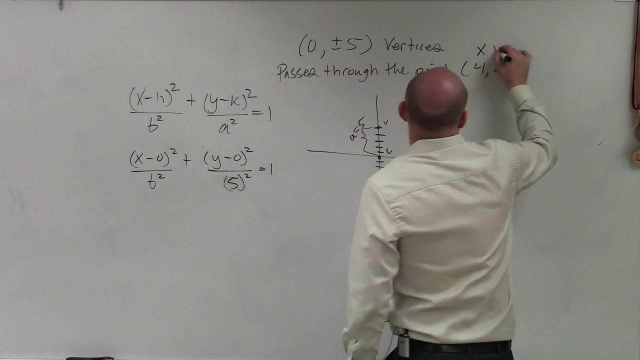 The only thing. y represents the distance from the center to my co-vertice. Do I have any information on my center to my co-vertice? No, And I don't know what my foci is for c, because usually we have the information for a and c, then we find b, But I don't have any information for the foci either. I do have information, though, on a random point that is on my ellipse, So I can plug that in for x and y. So now let's go ahead and do that. So I have. 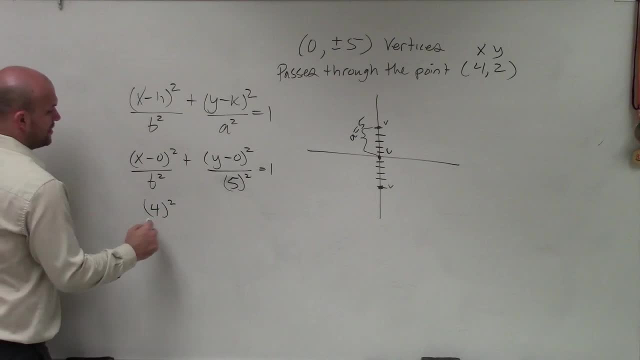 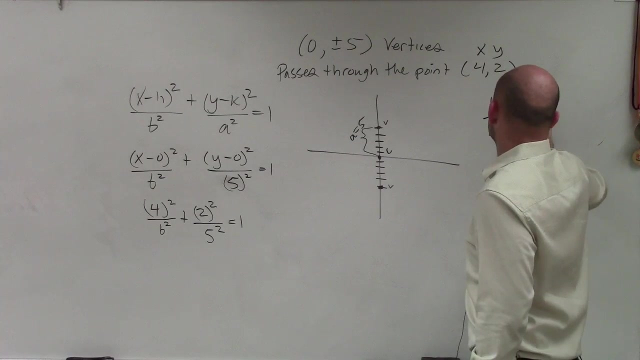 4 minus 0 is just 4 squared over b, squared plus 2 minus 0. squared over 5 squared equals 1.. So now let's just go ahead and fix this. That's 16 over b squared equals 4 over plus 4 over 25 equals 1.. 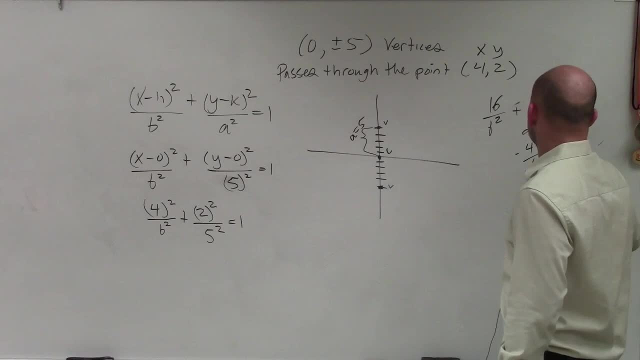 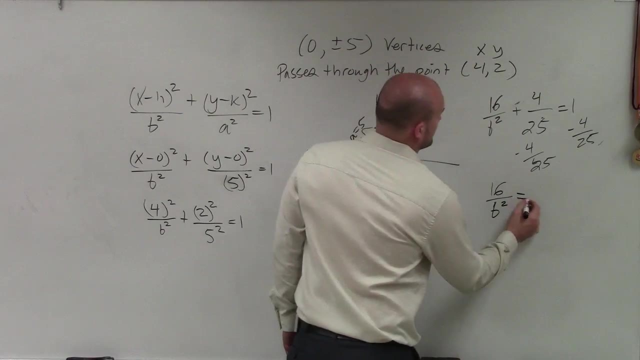 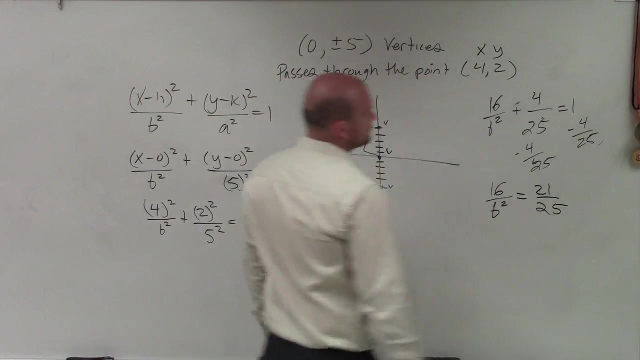 To solve for b squared, I'll subtract 4 over 25.. So I have 16 over b. squared is going to equal 21 over 25.. Yes, Anybody need me to? No, no, no, Is that correct? 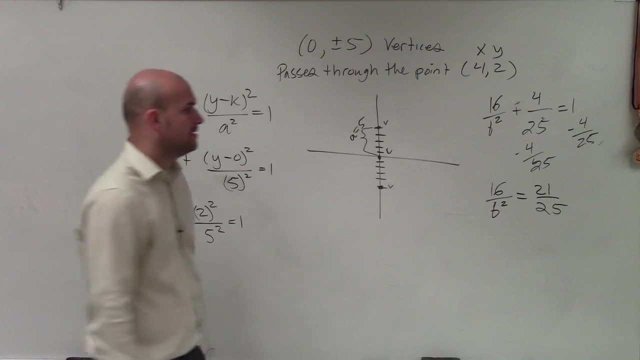 Because you changed the 1 to 25 over 25? OK, Now you could do this a couple different ways. One way to do it is just be to cross multiply: 21b squared equals 16 times 25, which I do not know. 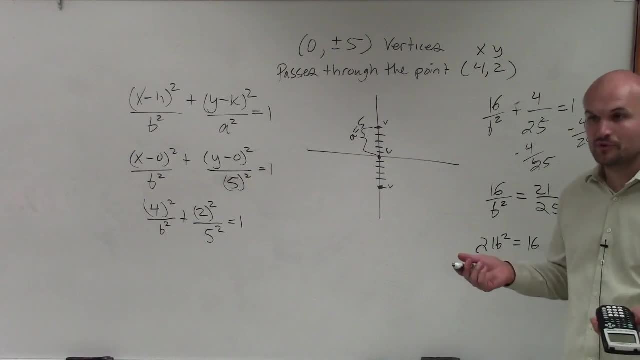 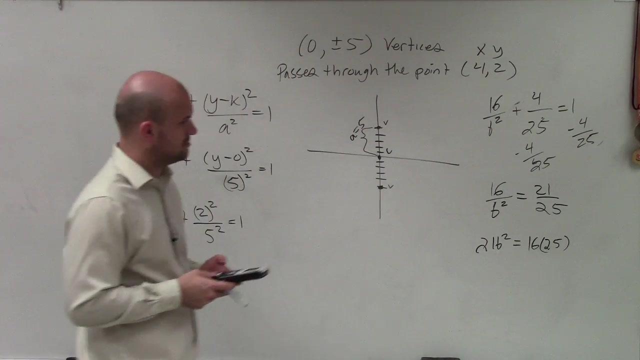 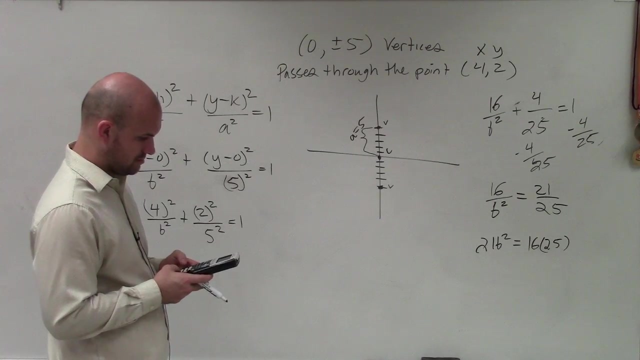 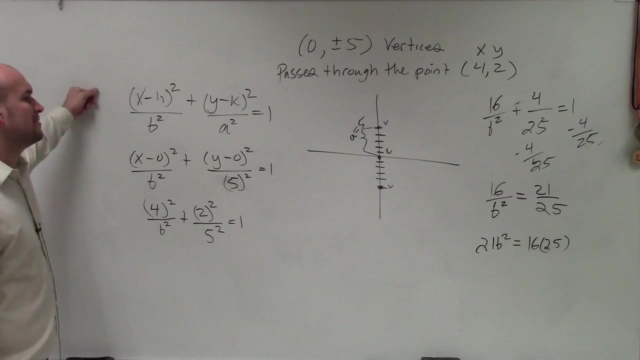 16 times 25 is 400.. And the square root, or so that's times 25.. And then divide that by 21.. Ooh, That's not good. I don't remember getting that answer. What happened? 16,, that's 4 over 25..